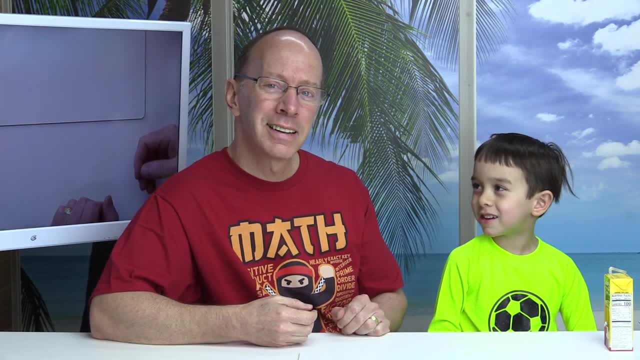 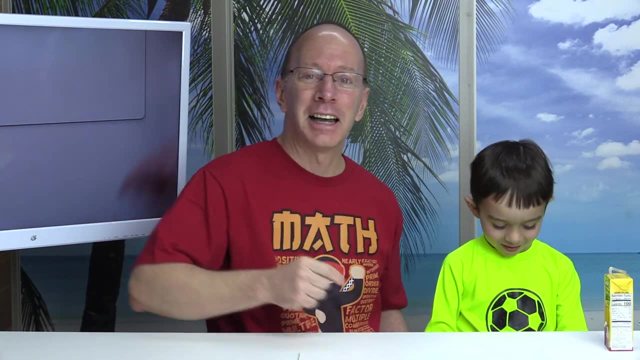 Hi Lucas. Hey, do you know what time it is? Um, it's almost lunchtime. Lunchtime. What time is lunchtime? It's 12 o'clock, 12 o'clock. Hey, on today's show we are going to be. 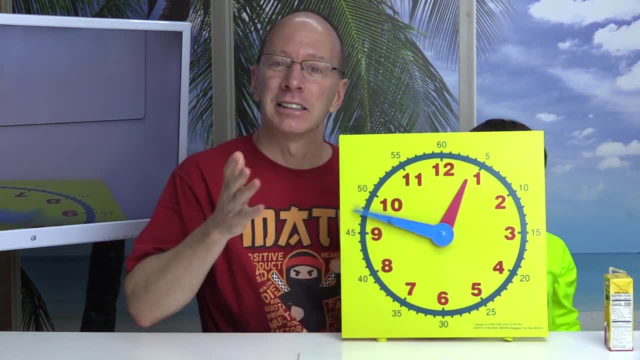 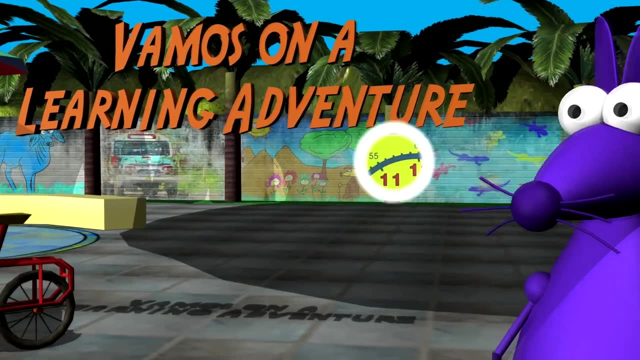 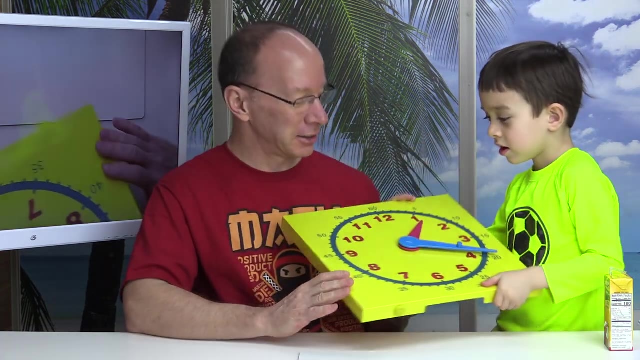 learning about the clock and telling time to the nearest hour. Stay tuned, Hey. welcome back to the show. Today we're going to be talking about how to tell time on a clock to the nearest hour. On a clock there are How many hours are on? 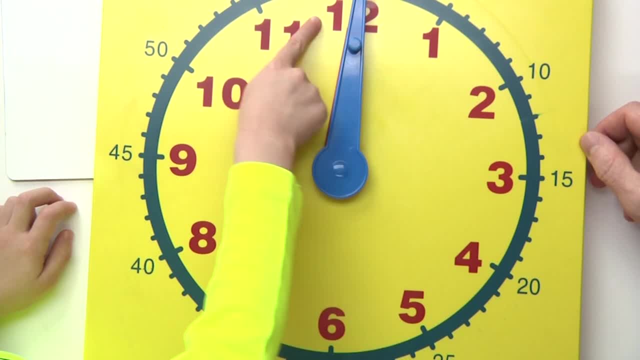 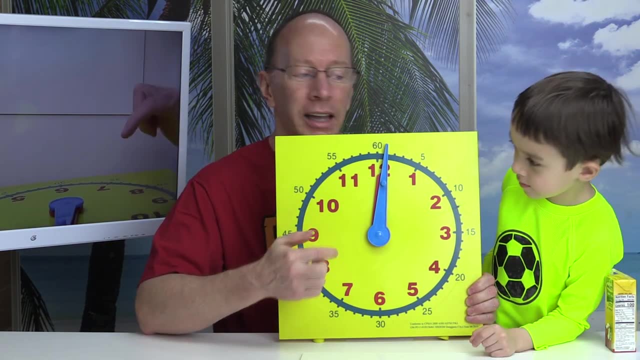 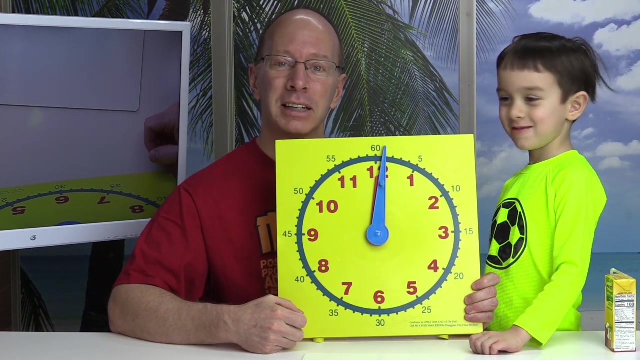 a clock, Um 12.. So, on a clock, there is 12 hours on a clock, And can you guess how many minutes are in an hour? Um an hour, There are 60 minutes in an hour. So for 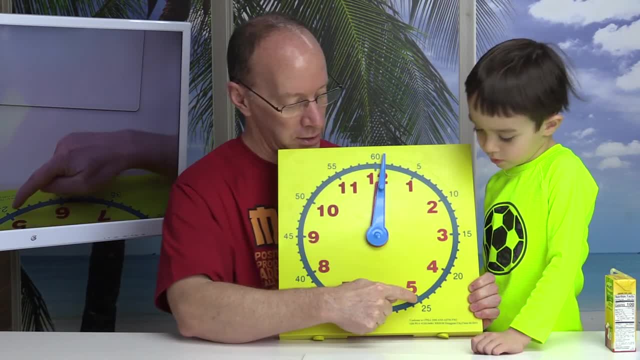 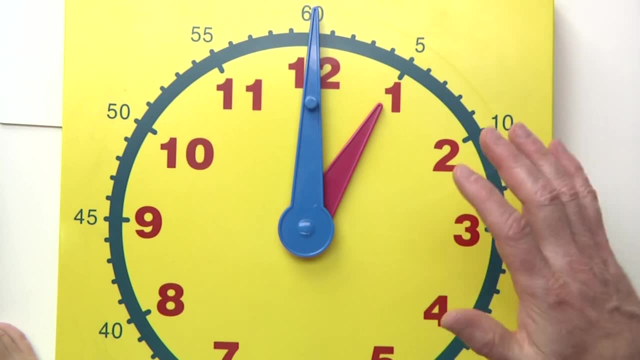 instance, here's 5,, 10,, 15,, 20,, 25,, 30,, 35,, 40,, 45,, 50,, 55, 60.. On a clock there are two hands. There is the hour. 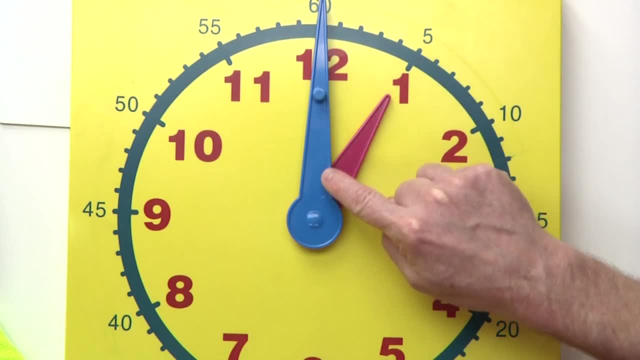 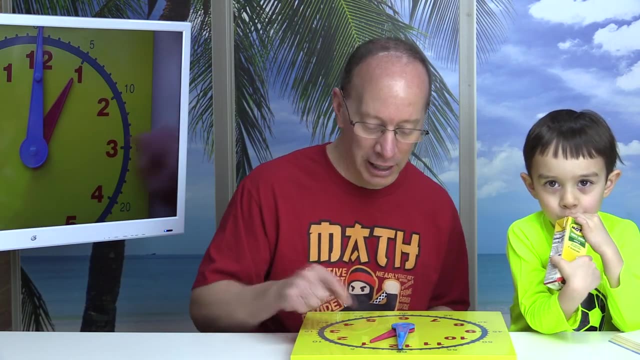 hand. that is the short hand right here, Lucas, and the long hand right here is the minute hand, And I like to say that the long hand is the man hand and the short one is the lady hand. So, um, my mom always taught me that. 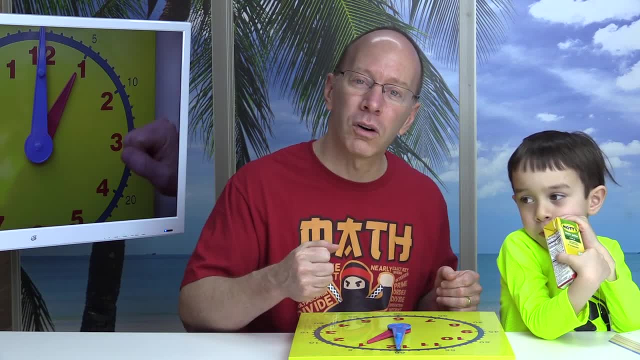 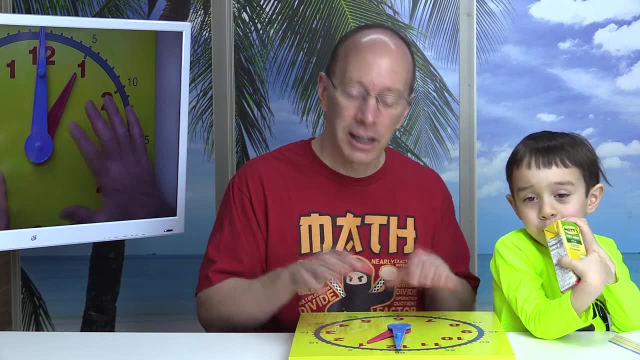 when I go into by a door that I always hold the door open for a lady because a lady needs to go first. So when we read a clock we always look at the lady hand first. We always say what this one is. 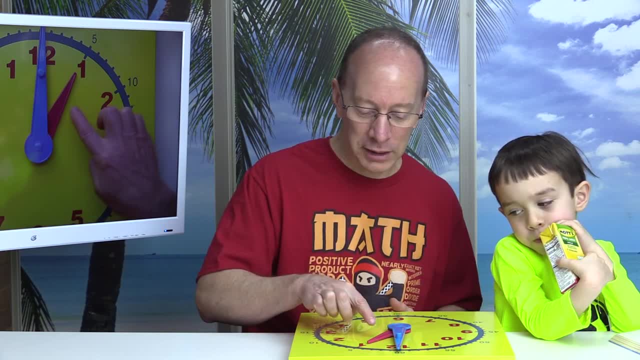 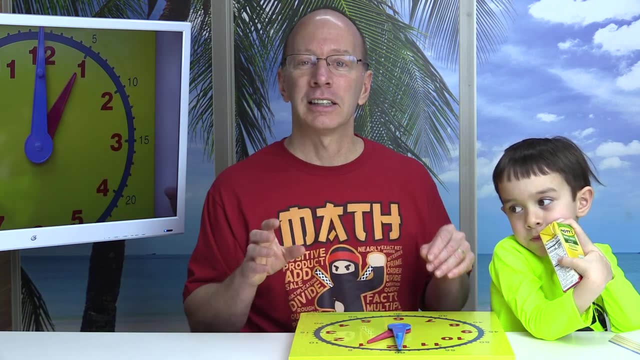 first, because ladies come first. So, for instance, right now, um, the minute hand is all the way to the top, and so we're just going to learn about telling time to the nearest hour today. So can you tell me? 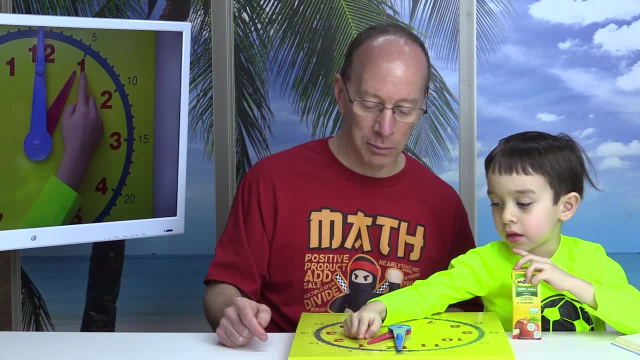 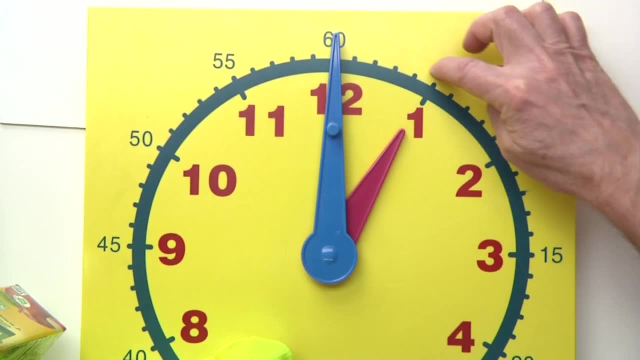 which number is the lady hand, the hour hand pointing to Um? the one, The one that is correct, And the five. Well, that's, that's nice that you noticed the five right here, and these are actually minutes. 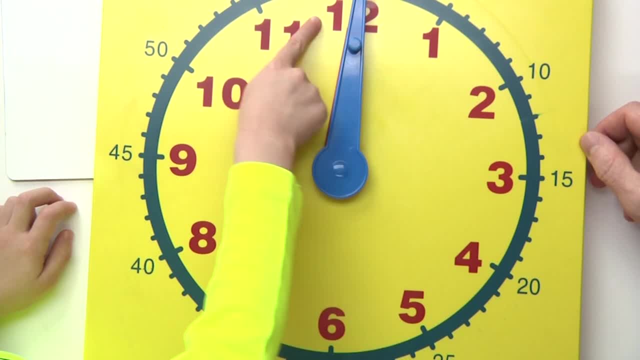 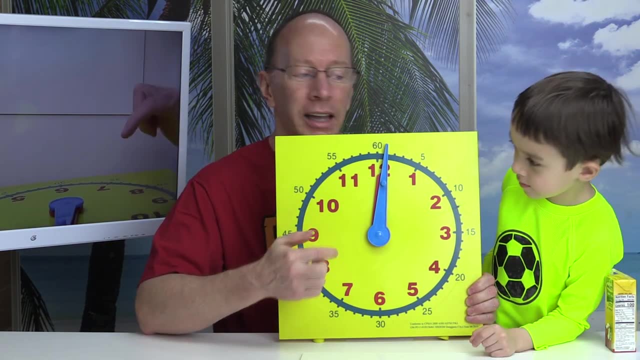 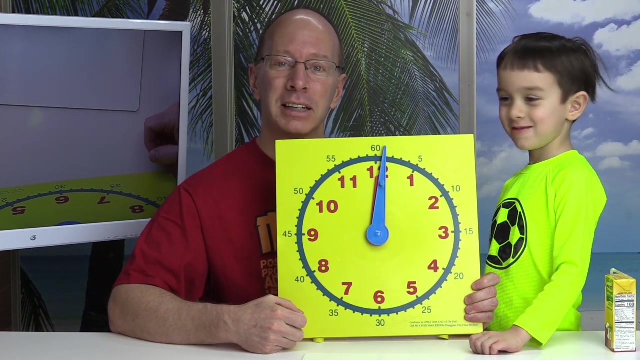 a clock, Um 12.. So, on a clock, there is 12 hours on a clock, And can you guess how many minutes are in an hour? Um an hour, There are 60 minutes in an hour. So for 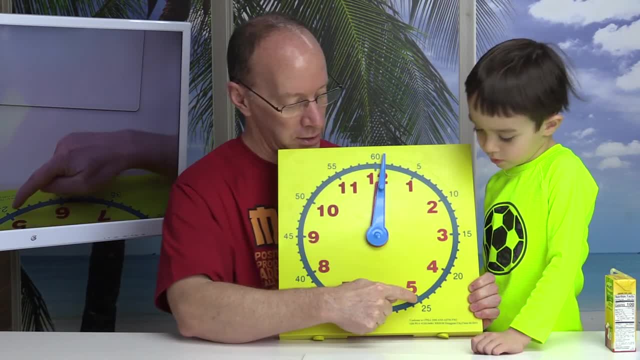 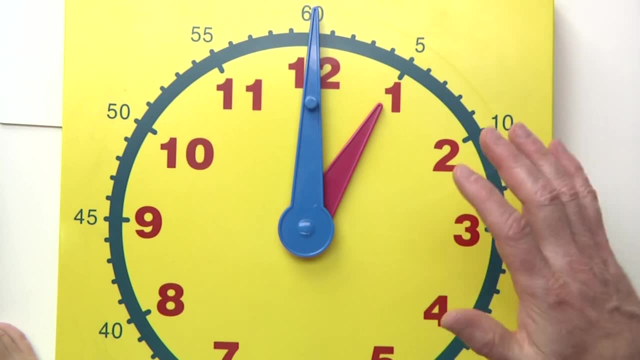 instance, here's 5,, 10,, 15,, 20,, 25,, 30,, 35,, 40,, 45,, 50,, 55, 60.. On a clock there are two hands. There is the hour. 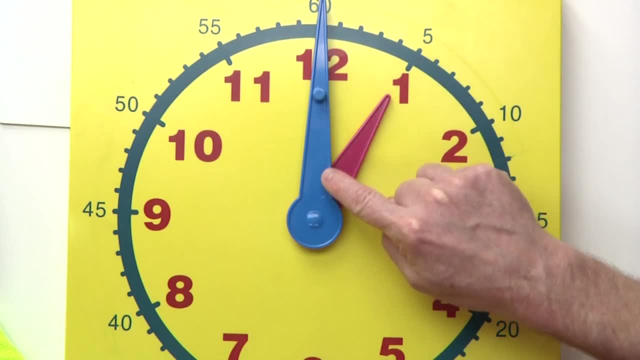 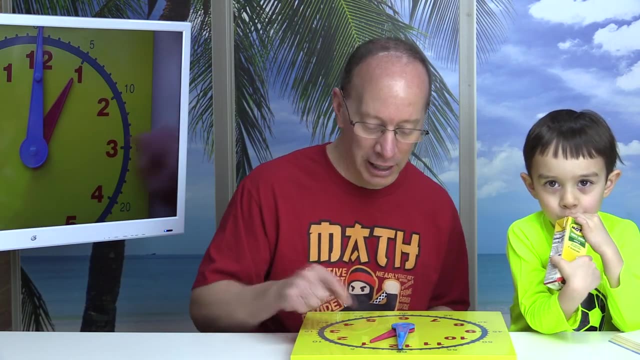 hand. that is the short hand right here, Lucas, and the long hand right here is the minute hand, And I like to say that the long hand is the man hand and the short one is the lady hand. So, um, my mom always taught me that. 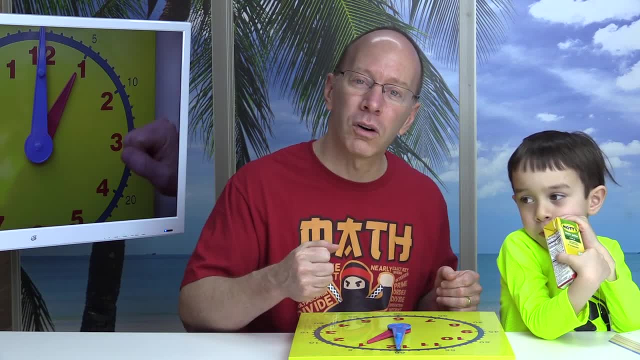 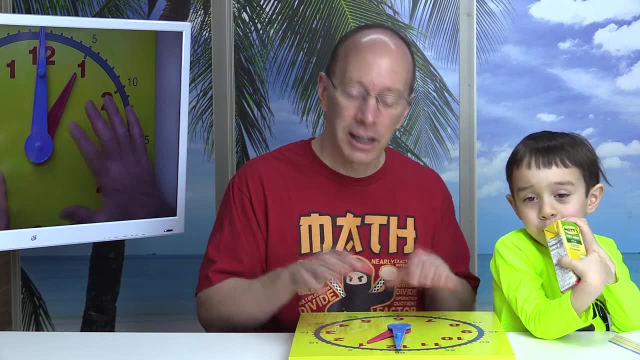 when I go into by a door that I always hold the door open for a lady because a lady needs to go first. So when we read a clock we always look at the lady hand first. We always say what this one is. 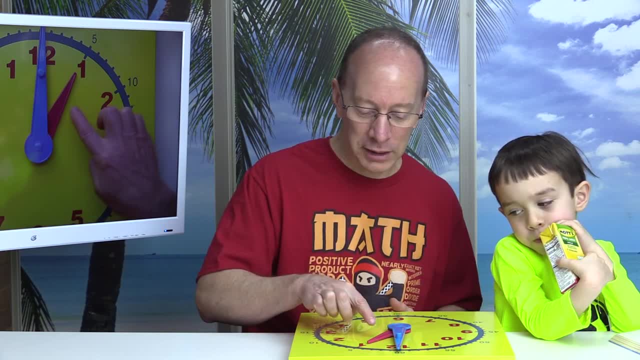 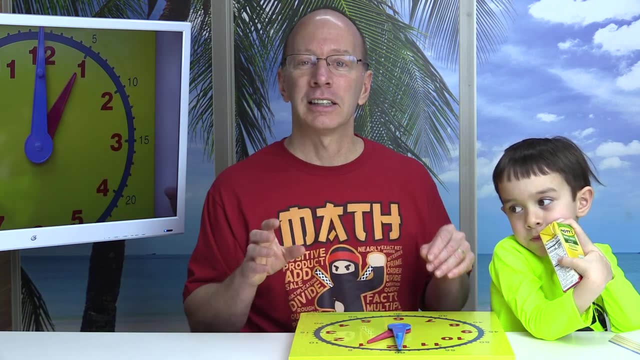 first, because ladies come first. So, for instance, right now, um, the minute hand is all the way to the top, and so we're just going to learn about telling time to the nearest hour today. So can you tell me? 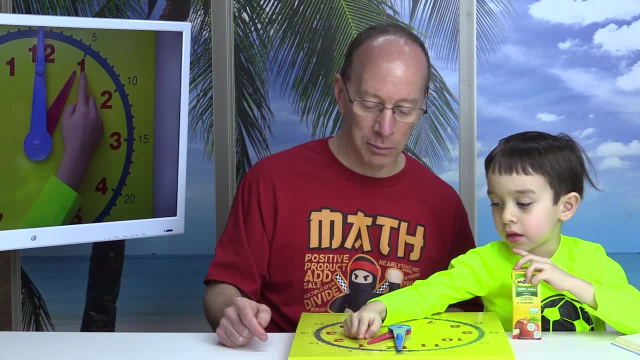 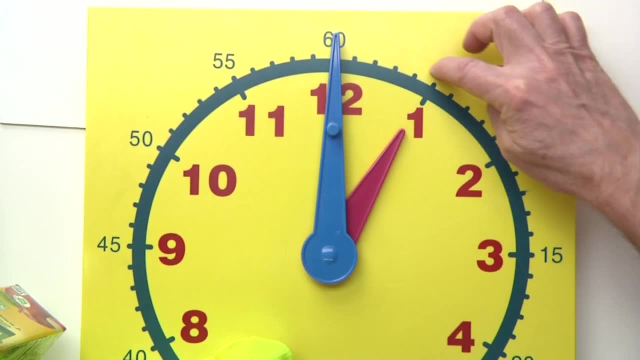 which number is the lady hand, the hour hand pointing to Um? the one, The one that is correct, And the five. Well, that's, that's nice that you noticed the five right here, and these are actually minutes. 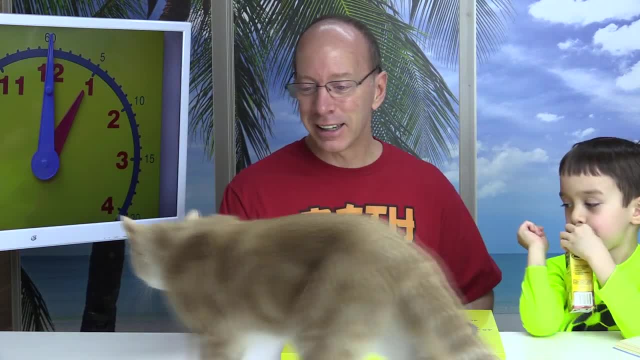 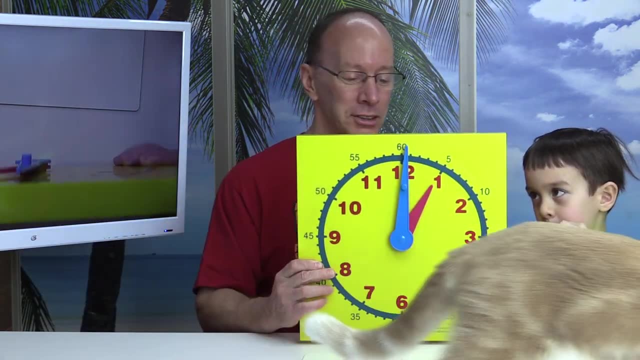 And there are sixty minutes in an hour. Hello kitty, Our kitty loves to learn our math lessons all the time and wants to learn math with us. So right now, Lucas, it is one o'clock. Can you tell me what time it is now? 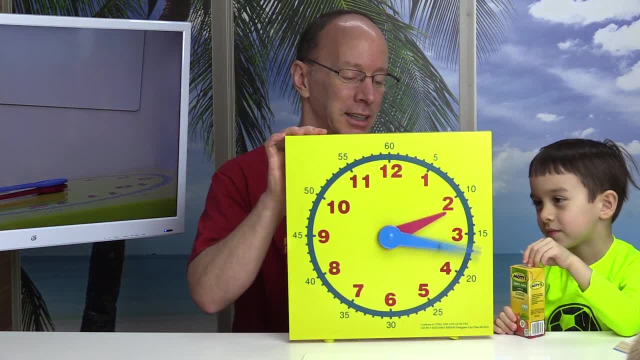 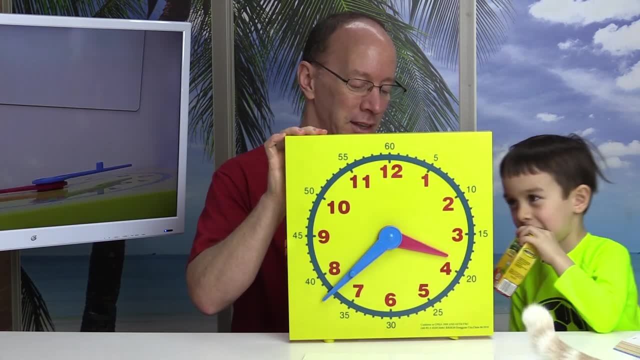 Um two o'clock, Two o'clock. Can you tell me what time it is now Um three o'clock, Three o'clock. Now let's put the minute hand. the minute hand or the man hand always has to. 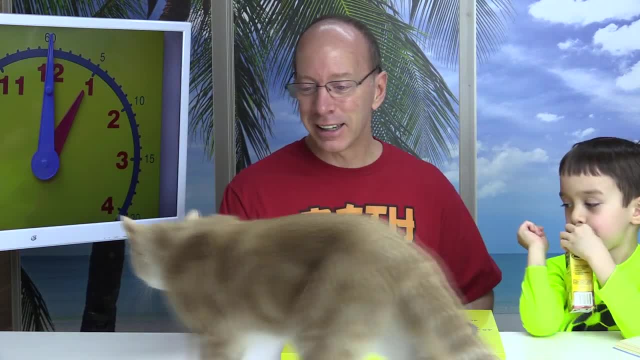 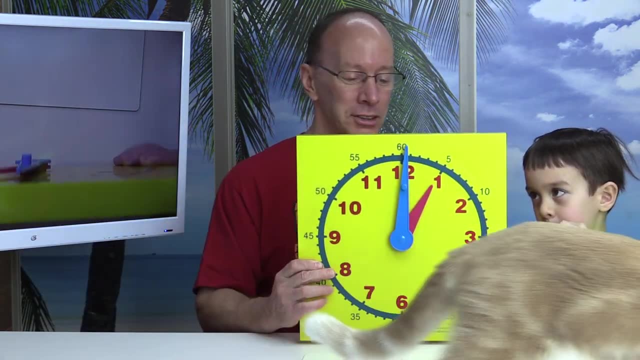 And there are sixty minutes in an hour. Hello kitty, Our kitty loves to learn our math lessons all the time and wants to learn math with us. So right now, Lucas, it is one o'clock. Can you tell me what time it is now? 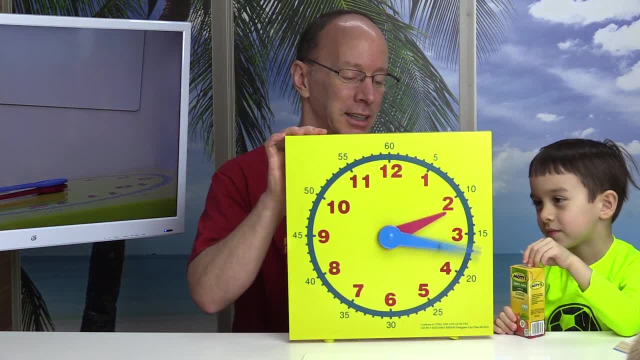 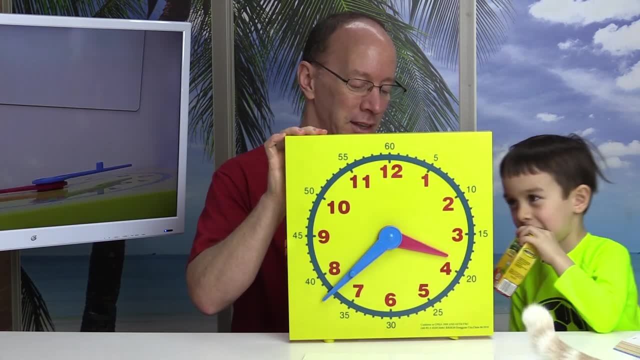 Um two o'clock, Two o'clock. Can you tell me what time it is now Um three o'clock, Three o'clock. Now let's put the minute hand. the minute hand or the man hand always has to. 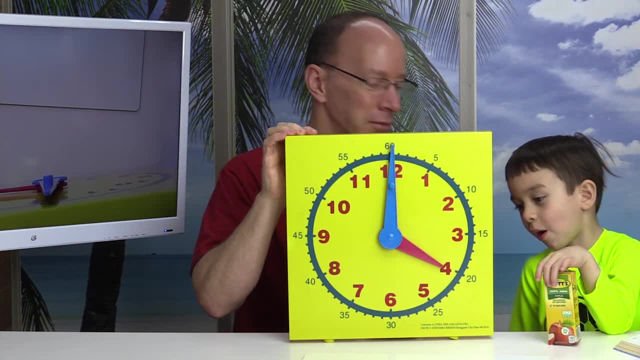 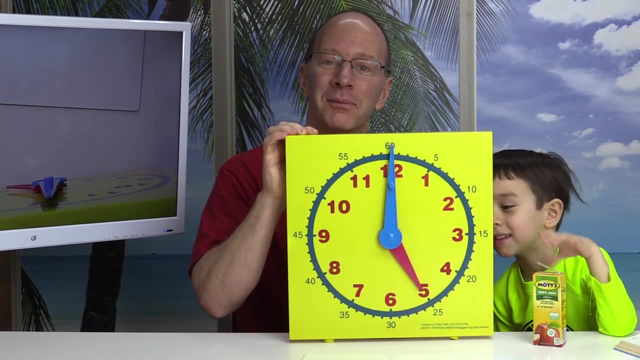 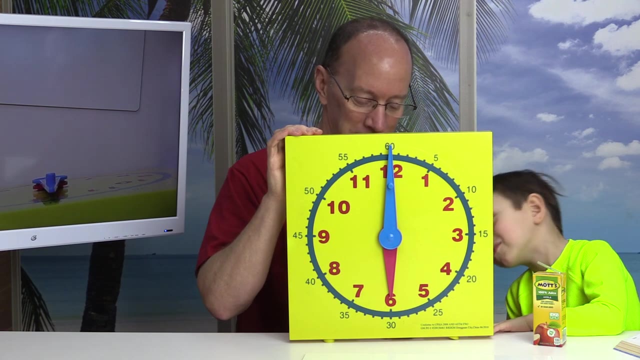 be at the very top there. What time is it now Four o'clock, Four o'clock. What time is it now Um five o'clock, Five o'clock. What time is it now? Six o'clock Now. this is a tricky one, because you're like 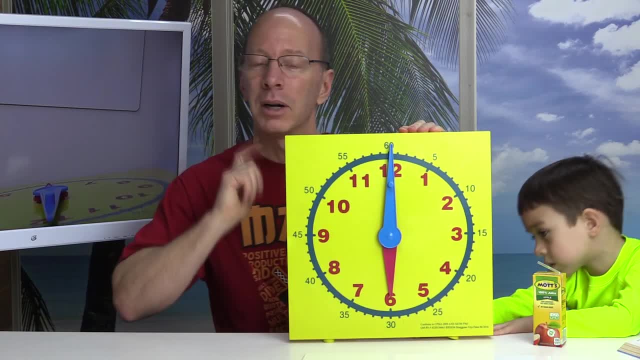 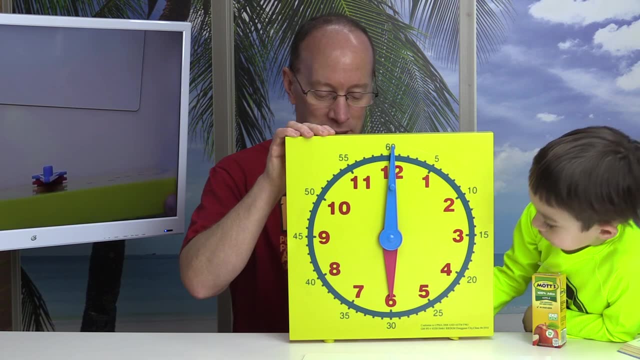 okay, this hand is pointing this way and this hand is pointing this way, but remember, always take a look at the lady hand first, the short hand first. That's the hour hand right here And that's six o'clock. Very good. 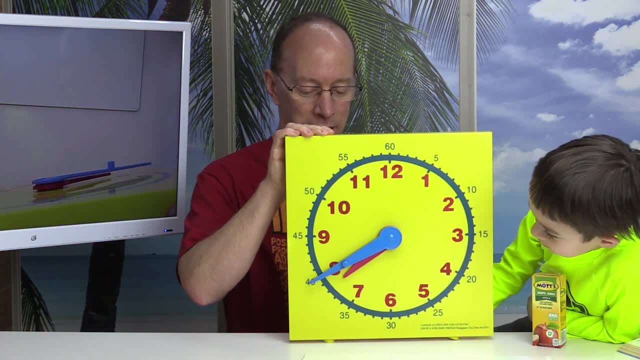 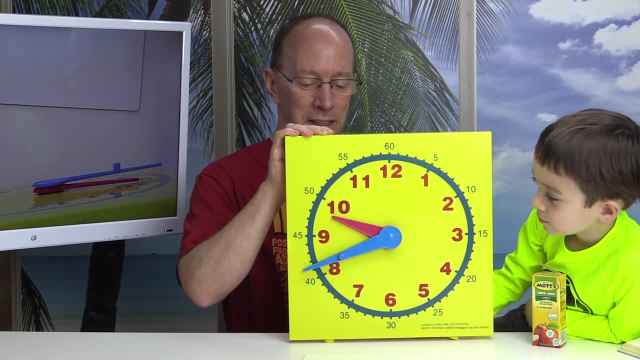 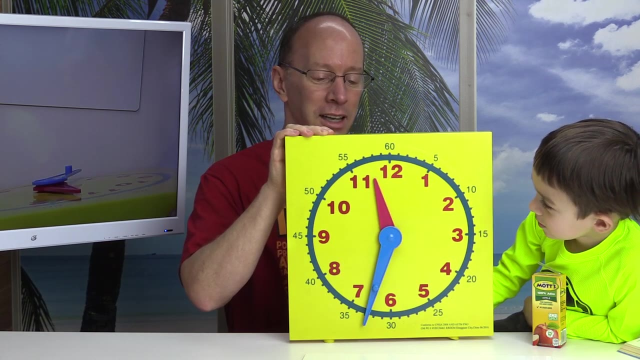 And we have Seven o'clock. Okay, You're doing good. Eight o'clock, Very good. Nine o'clock, Very good. Ten o'clock, Ten o'clock, Eleven o'clock. Eleven o'clock Um twelve o'clock. Twelve o'clock. 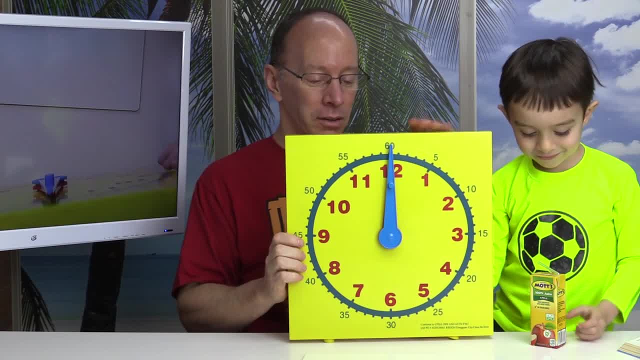 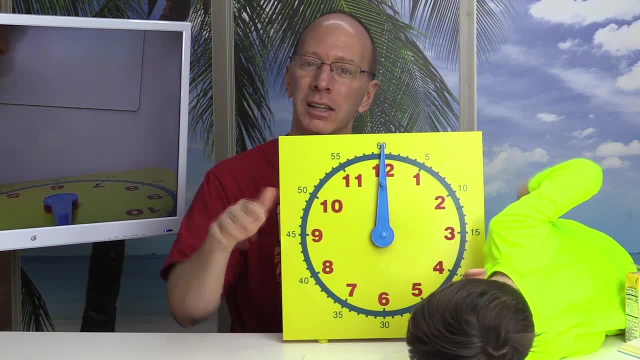 That's when we are going to be eating lunch. Now there are twelve hours on this clock, but there are also twenty-four hours in a day and we're going to be talking about that more on another show, So I'm going to give you. 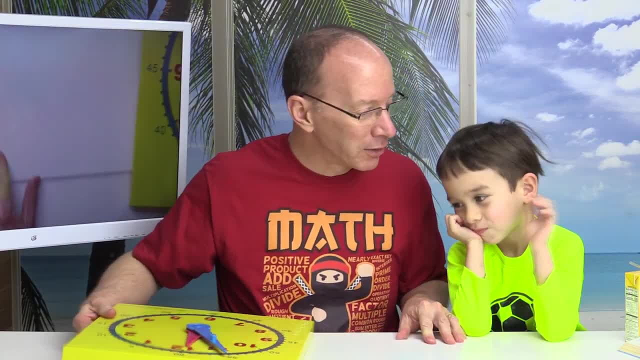 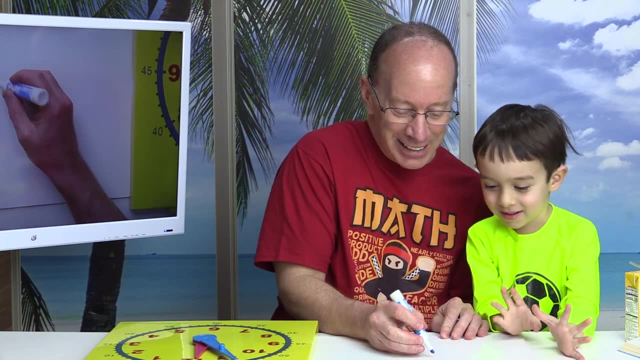 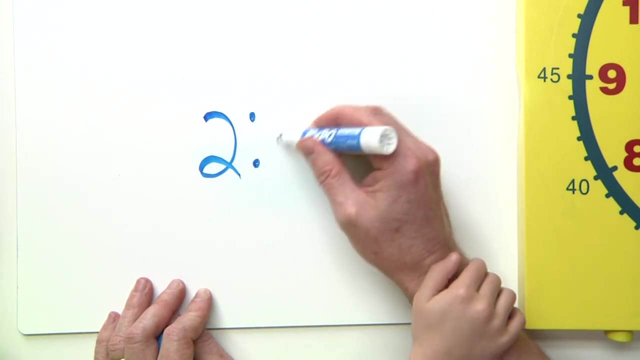 a challenge here. okay, Lucas, I am going to be writing down a number here. Aha, Okay, You're going to be similar. This is how you write: two o'clock With a two and two little dots right here. 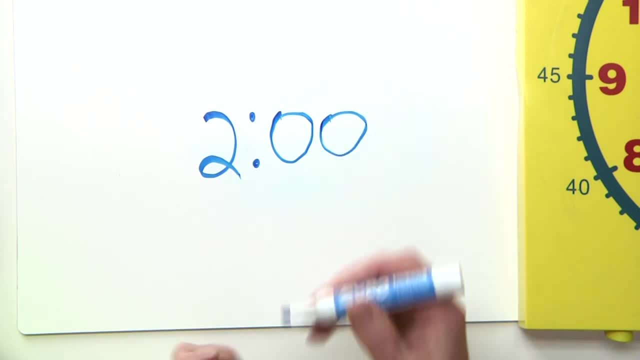 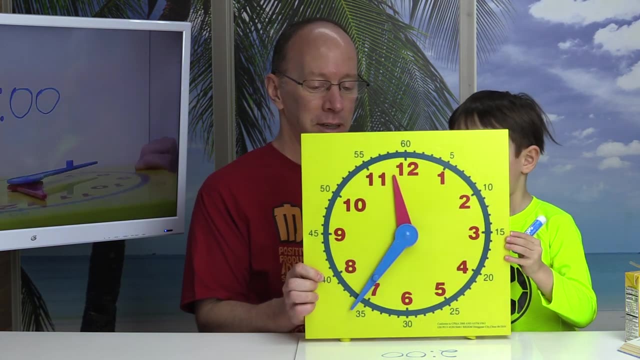 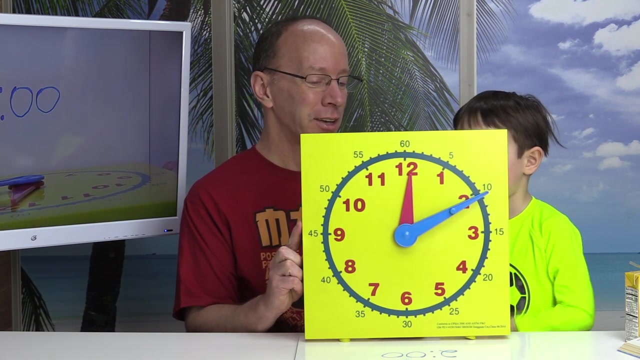 a zero and a zero. Can you make a two o'clock right here on this, one for me? Can you move the dial there for me? Go the other way, Keep it going. Okay, Is he right here? Let's check. 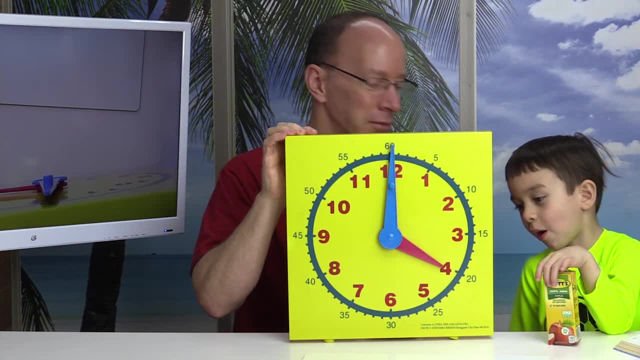 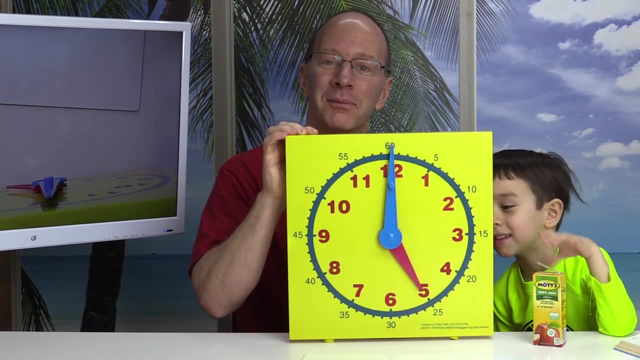 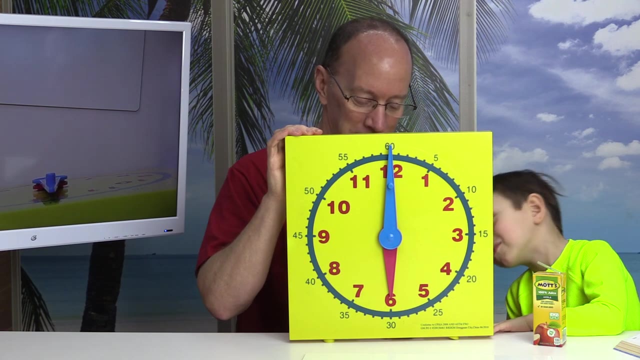 be at the very top there. What time is it now Four o'clock, Four o'clock. What time is it now Um five o'clock, Five o'clock. What time is it now? Six o'clock Now. this is a tricky one, because you're like 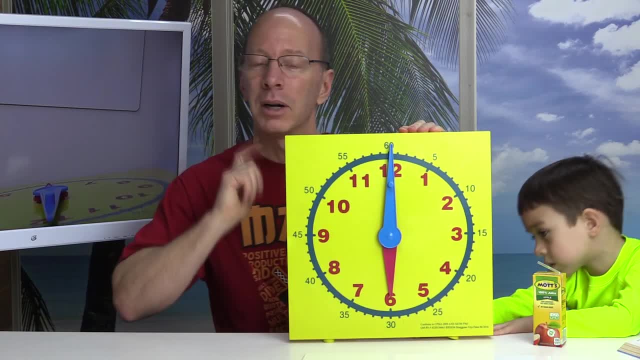 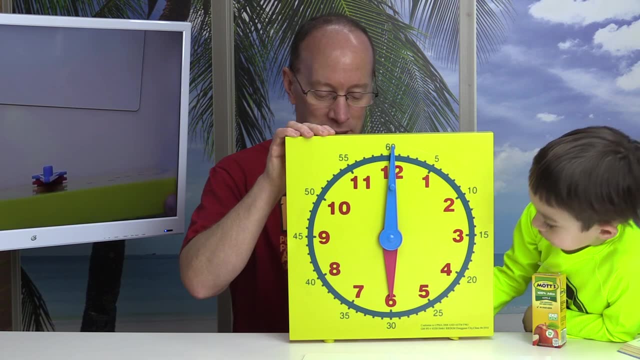 okay, this hand is pointing this way and this hand is pointing this way, but remember, always take a look at the lady hand first, the short hand first. That's the hour hand right here And that's six o'clock. Very good. 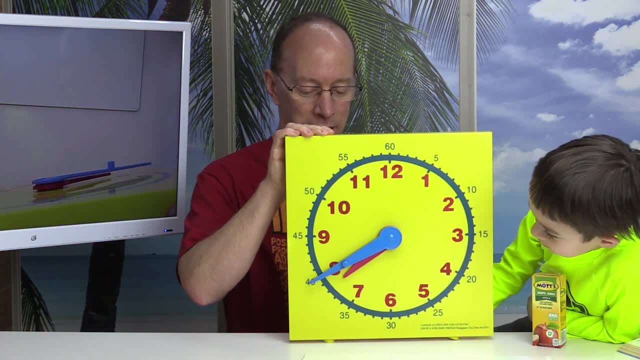 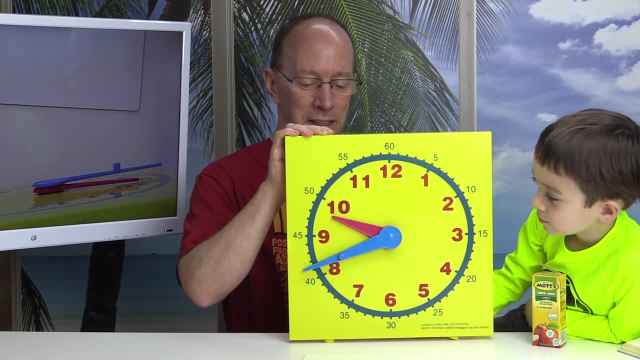 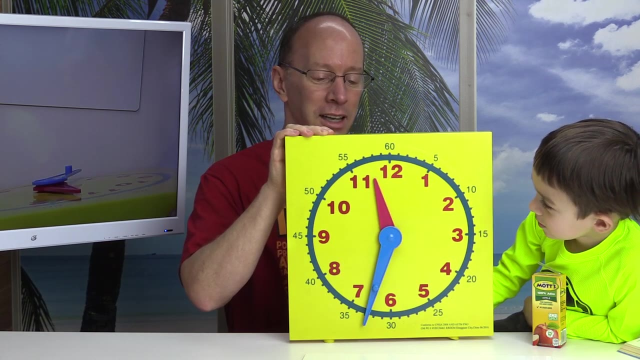 And we have Seven o'clock. Okay, You're doing good. Eight o'clock, Very good. Nine o'clock, Very good. Ten o'clock, Ten o'clock, Eleven o'clock. Eleven o'clock Um twelve o'clock. Twelve o'clock. 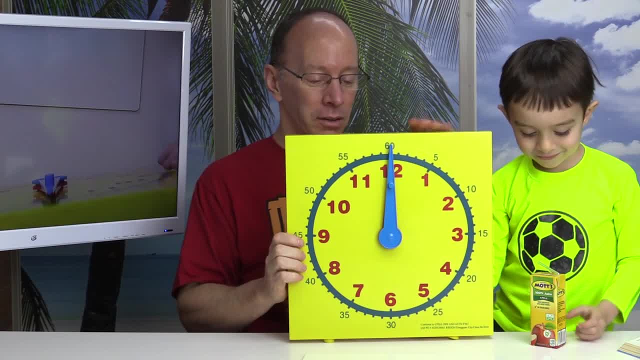 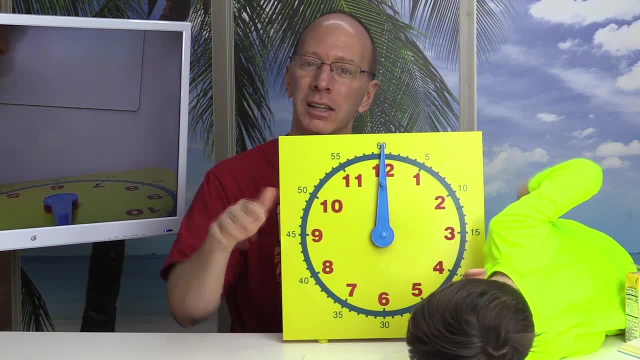 That's when we are going to be eating lunch. Now there are twelve hours on this clock, but there are also twenty-four hours in a day and we're going to be talking about that more on another show, So I'm going to give you. 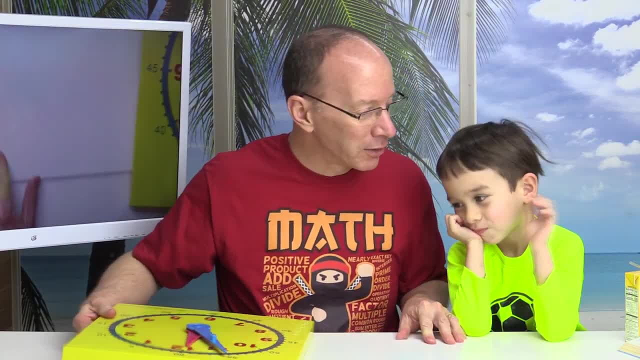 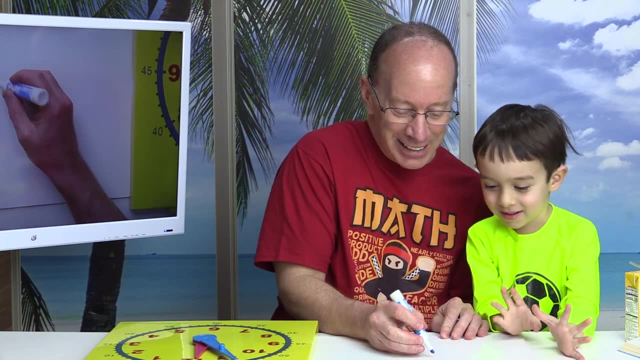 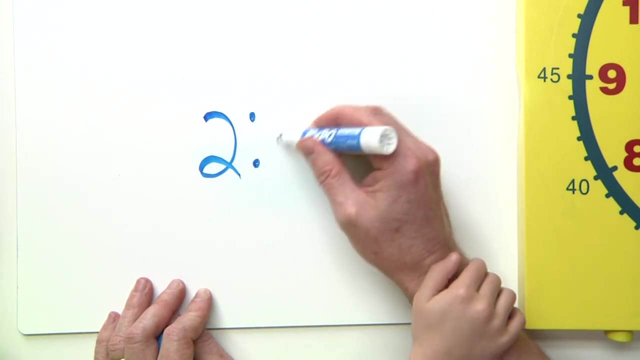 a challenge here. okay, Lucas, I am going to be writing down a number here. Aha, Okay, You're going to be similar. This is how you write: two o'clock With a two and two little dots right here. 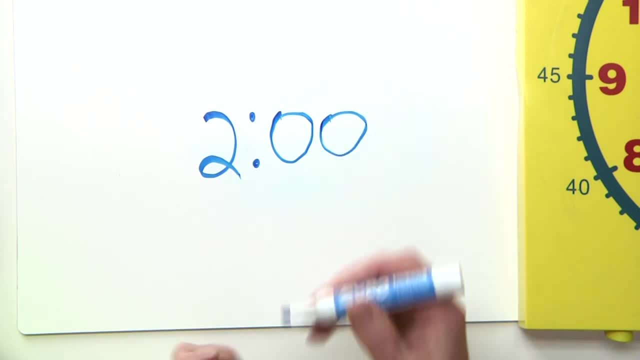 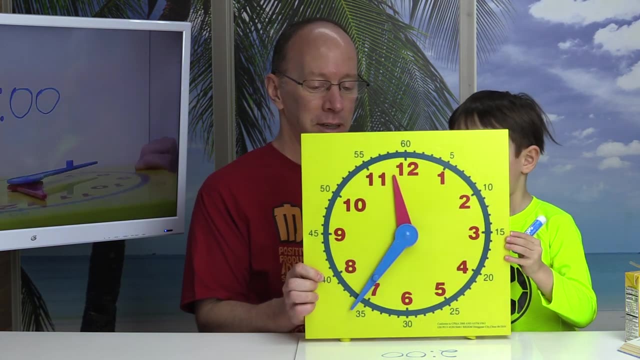 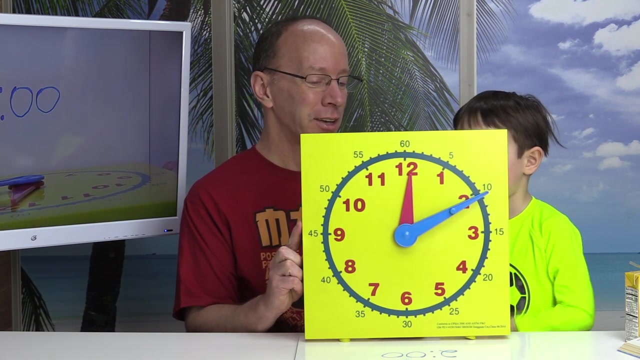 a zero and a zero. Can you make a two o'clock right here on this, one for me? Can you move the dial there for me? Go the other way, Keep it going. Okay, Is he right here? Let's check. 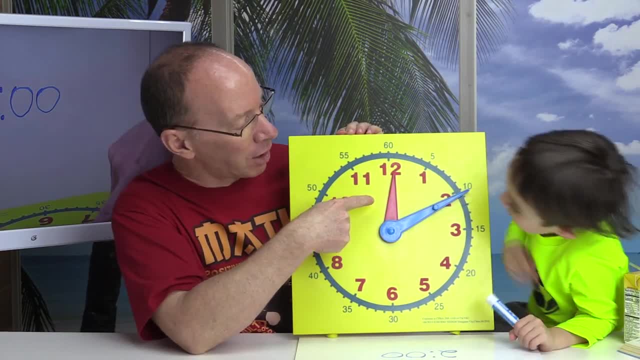 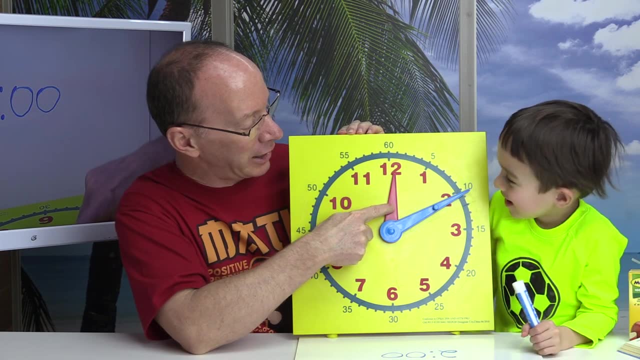 Alright, Which one are you supposed to always read first? Pick hand. Nope, The lady hand. remember The lady hand. So where is the lady hand supposed to be pointing to The two? The two, So that's okay, We always. 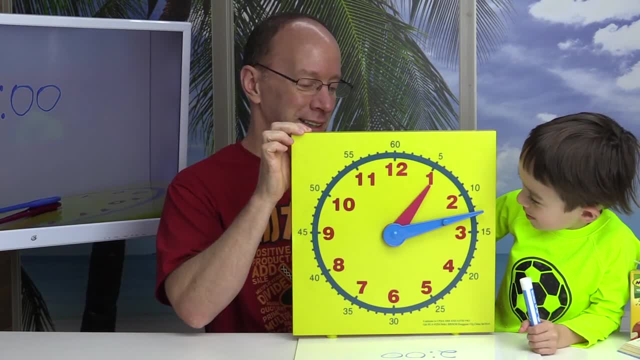 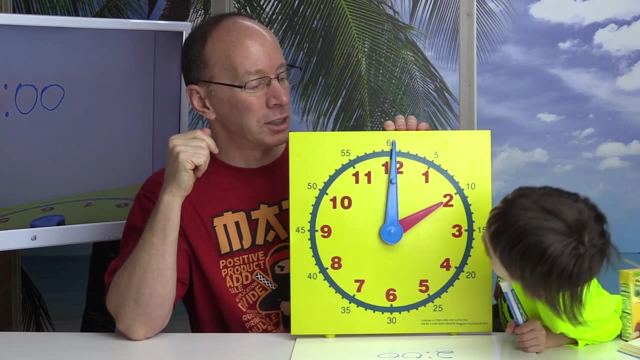 learn best from mistakes. I'm going to fix it up. Let me fix it up, That's better. Okay, Now read the lady hand or the hour hand first. Which number is it on? Two, The two, It is two o'clock, Just what it says. 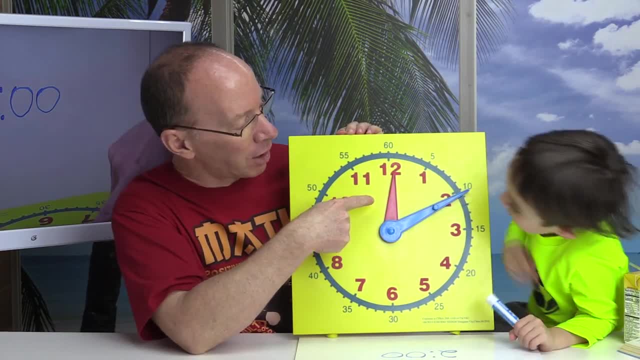 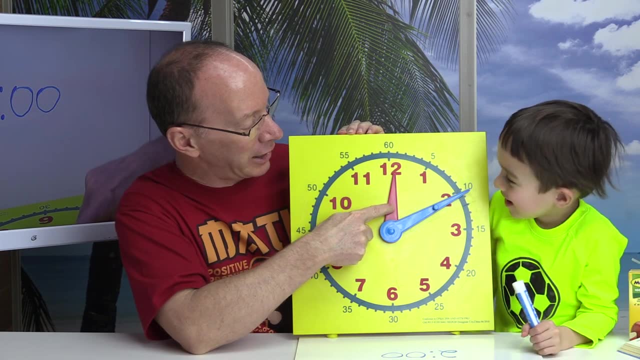 Alright, Which one are you supposed to always read first? Pick hand. Nope, The lady hand. remember The lady hand. So where is the lady hand supposed to be pointing to The two? The two, So that's okay, We always. 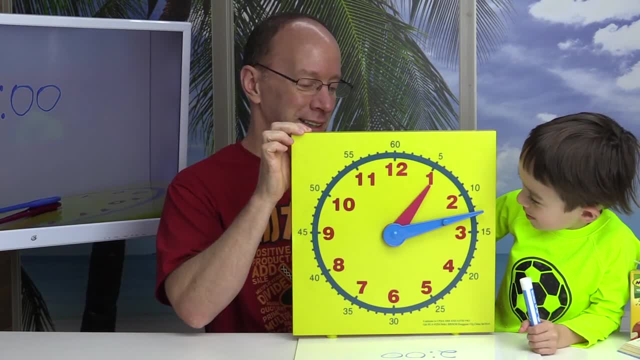 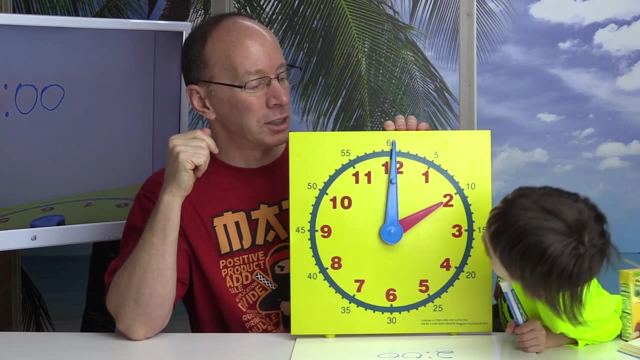 learn best from mistakes. I'm going to fix it up. Let me fix it up, That's better. Okay, Now read the lady hand or the hour hand first. Which number is it on? Two, The two, It is two o'clock, Just what it says. 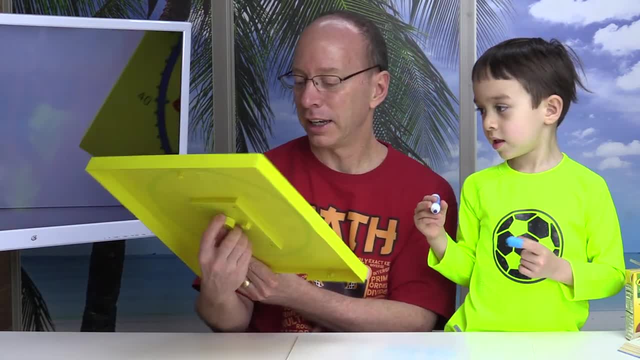 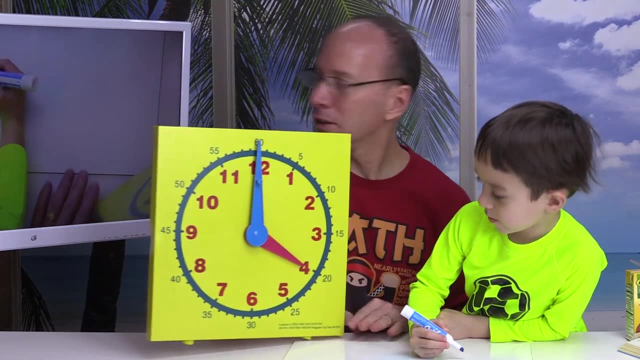 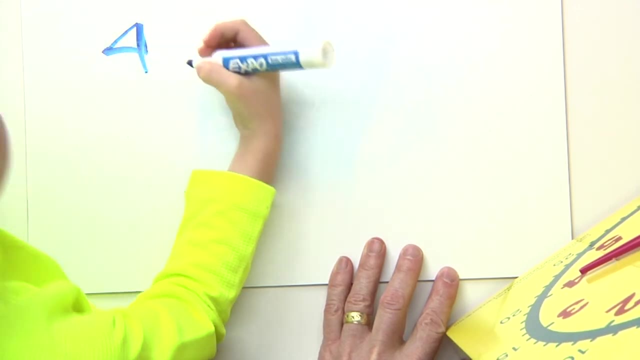 right here. Now I'm going to do another exercise for Lucas And he has to write down the time. Okay, Okay, Can you write down the time for me? Aha, Alright, Okay, Zero, Ah, I forgot. Yep, Two dots. 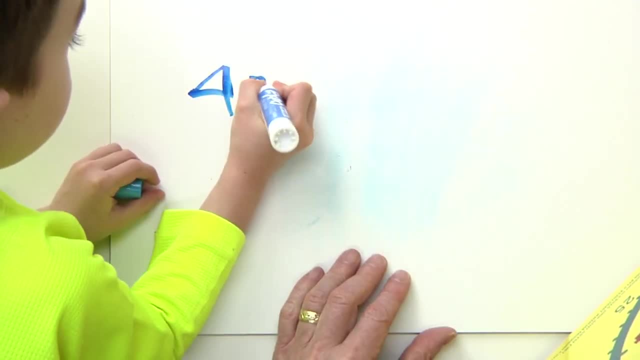 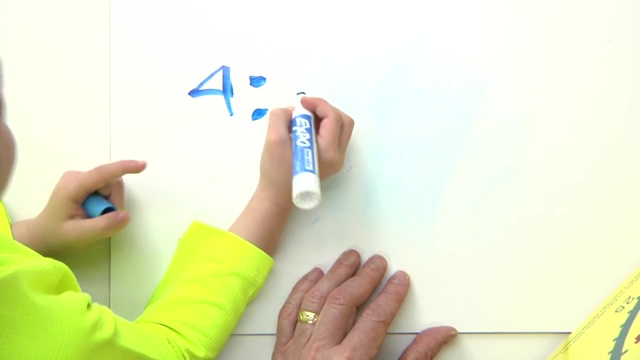 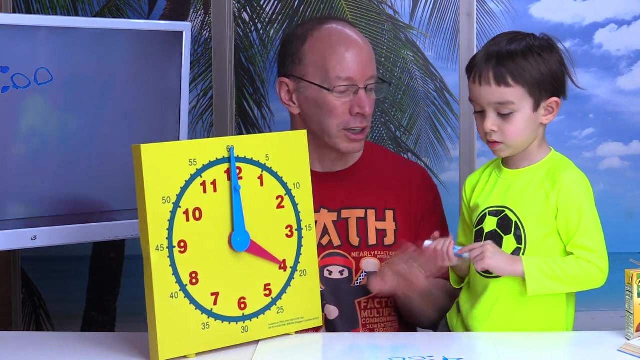 I forgot. Put another dot right there, Alright. And then two zeros, Alright. Am I giving you the answer? Okay, We'll do another one, so I won't give you the answer on the next one. That's awesome, Four o'clock, Alright. 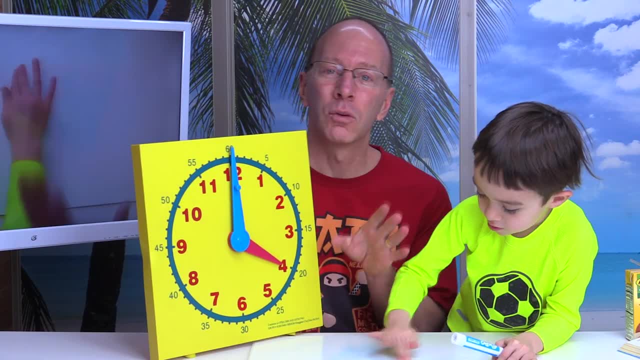 Let's go ahead and erase that. We're going to do another exercise And a lot of your workbooks that you might have at home. this is the type of exercise that you're going to be doing Now. I'm going to give you a clue. 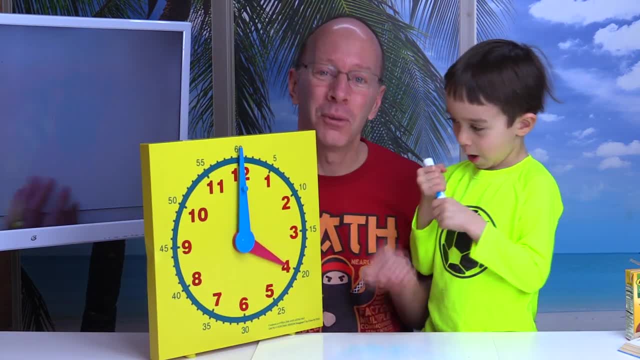 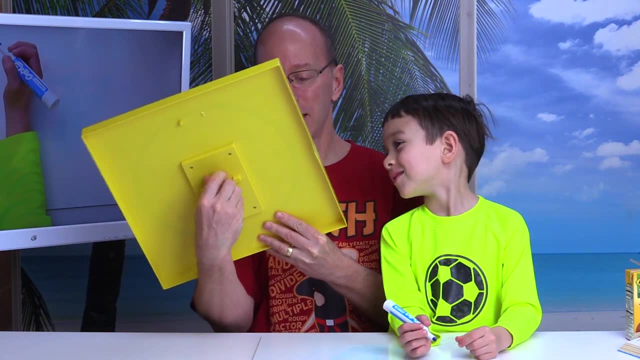 You're given the time and you're supposed to write down what time it is on the paper, So don't look, right now I'm going to make this a difficult one. Okay, Alright, Let's make this a really hard one for Lucas. 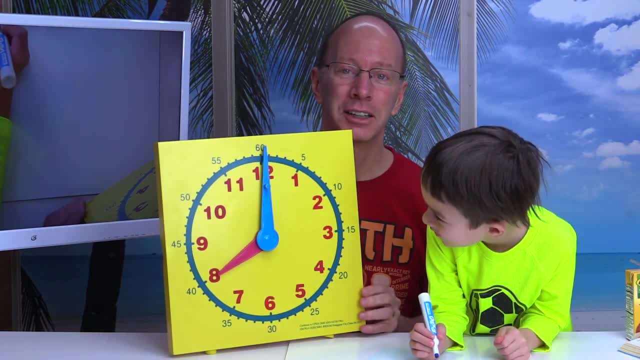 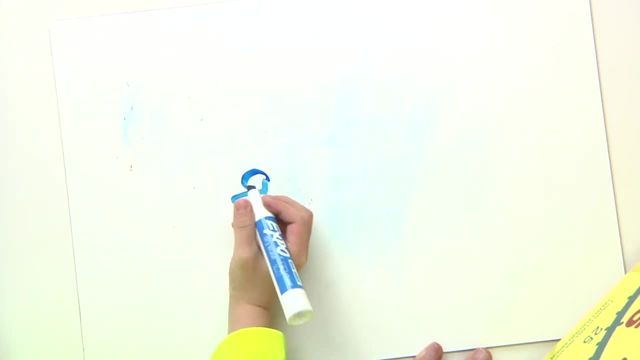 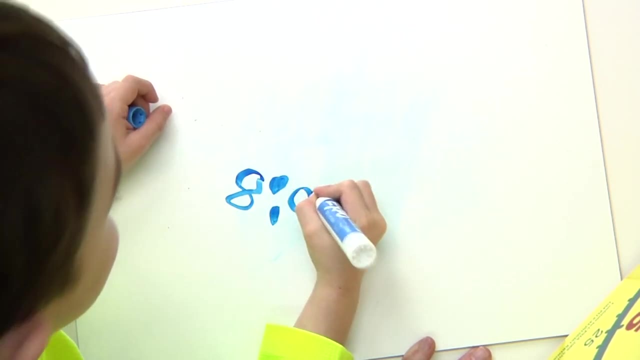 Okay, Lucas, I'm not going to give you any hints. Can you write down what time it is right here? Oh, I can do it. Our friends at home can see that. Okay, Okay, Awesome It is. 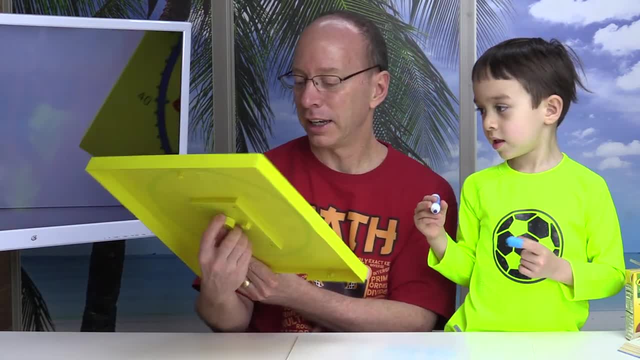 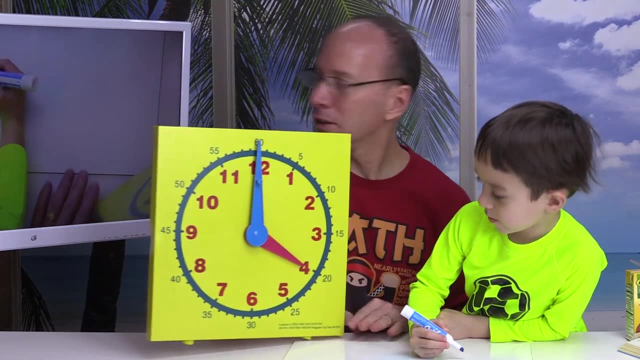 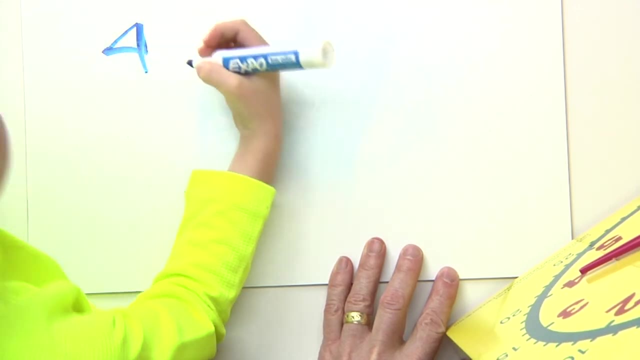 right here. Now I'm going to do another exercise for Lucas And he has to write down the time. Okay, Okay, Can you write down the time for me? Aha, Alright, Okay, Zero, Ah, I forgot. Yep, Two dots. 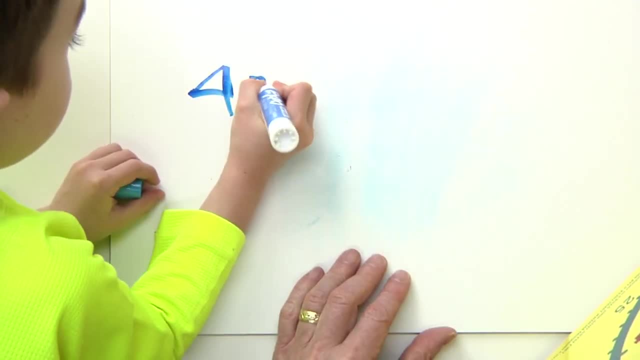 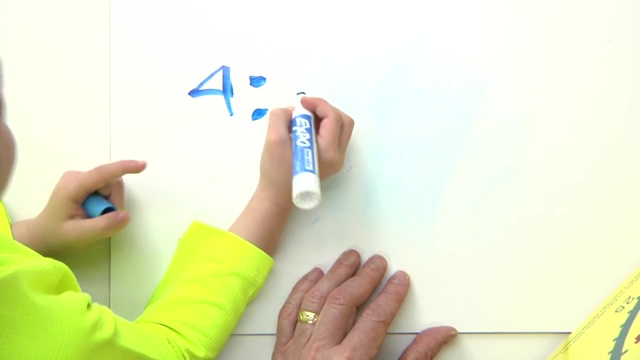 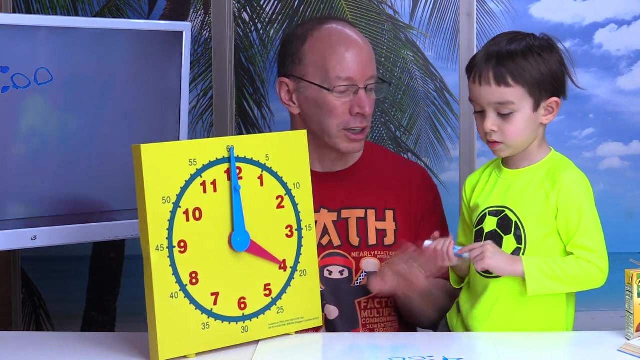 I forgot. Put another dot right there, Alright. And then two zeros, Alright. Am I giving you the answer? Okay, We'll do another one, so I won't give you the answer on the next one. That's awesome, Four o'clock, Alright. 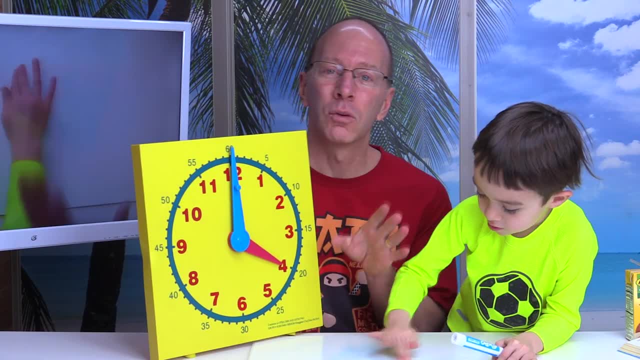 Let's go ahead and erase that. We're going to do another exercise And a lot of your workbooks that you might have at home. this is the type of exercise that you're going to be doing Now. I'm going to give you a clue. 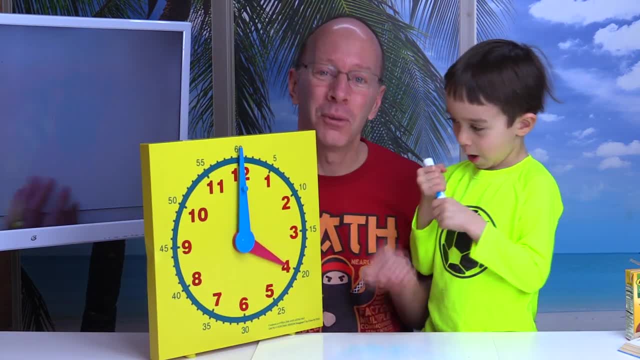 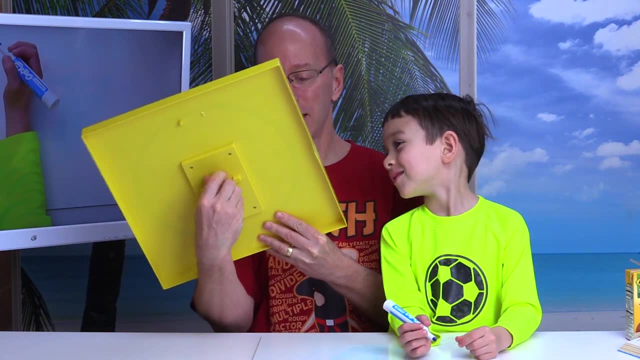 You're given the time and you're supposed to write down what time it is on the paper, So don't look, right now I'm going to make this a difficult one. Okay, Alright, Let's make this a really hard one for Lucas. 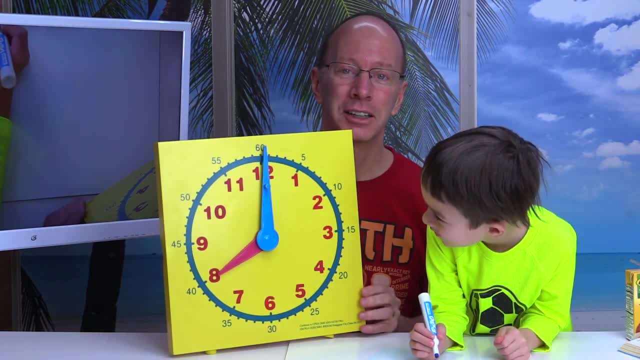 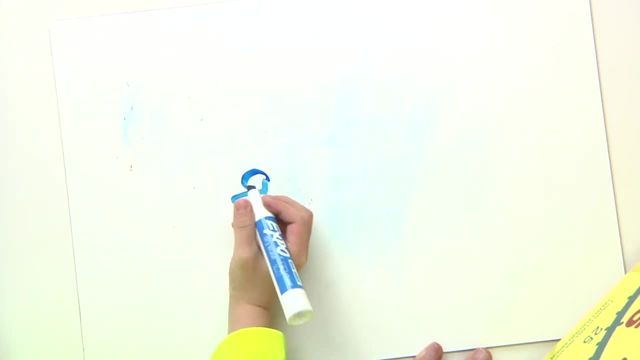 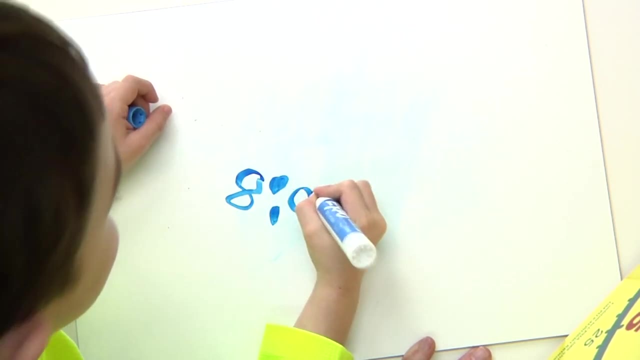 Okay, Lucas, I'm not going to give you any hints. Can you write down what time it is right here? Oh, I can do it. Our friends at home can see that. Okay, Okay, Awesome It is. 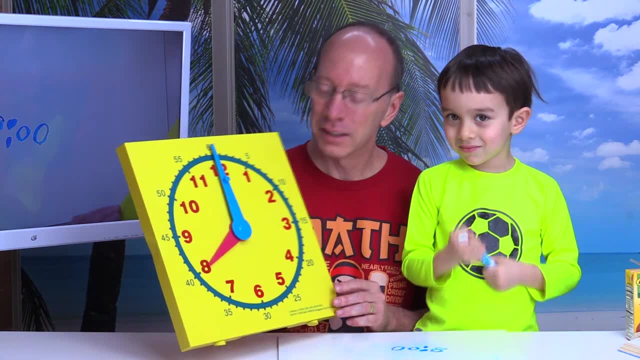 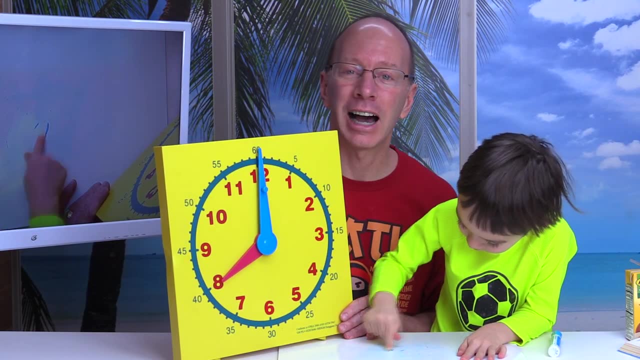 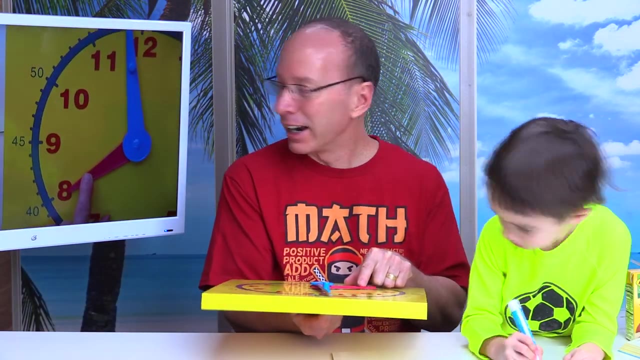 What time is it? Eight o'clock, Eight o'clock. This is a great exercise to do at home, And we're learning how to tell time to the nearest hour. Once again, I'm going to review. This is the. This is the hour hand. 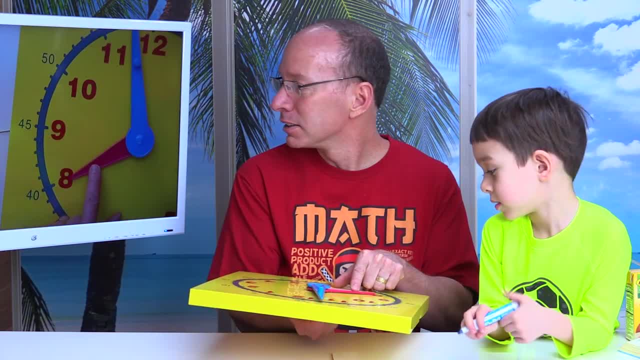 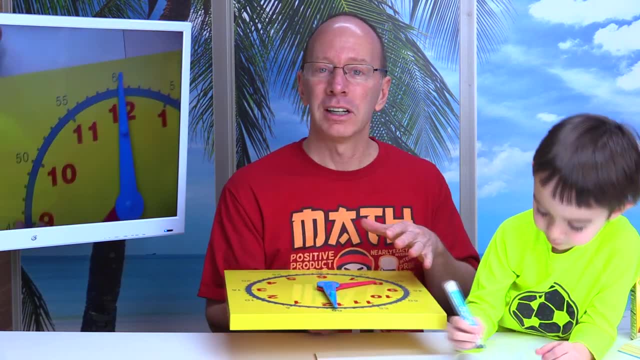 This is the minute hand. I like to say that this is the lady hand, because ladies always go first and so we want to always say the lady hand first, And when we're doing it to the nearest hour, we always want to make sure that the minute hand.